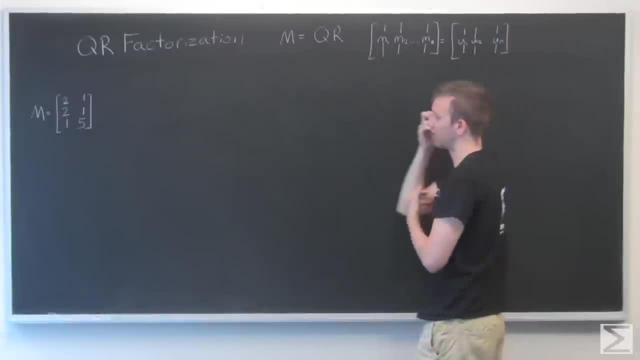 For however many columns that we want. Check the previous video for the Gram-Schmidt process on how exactly it is that we calculate this from these, But we're going to do it in this video anyway, so you get to see it again. 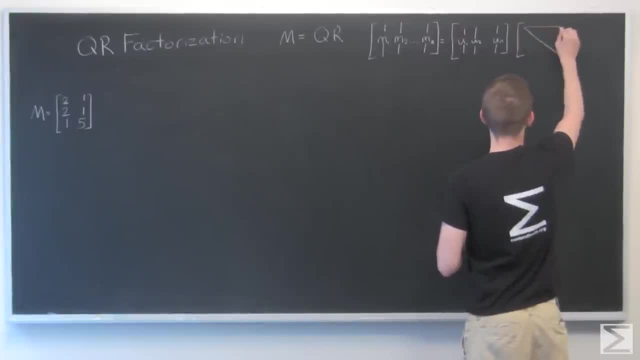 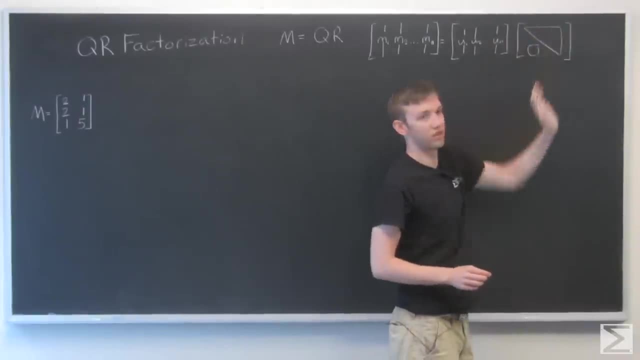 And finally, our R is some kind of upper triangular matrix that looks like that. So all zeros down here and then on the diagonal and above various numbers and things, That's R, And that's Q, And that's M, And that's our reference that we'll look at. 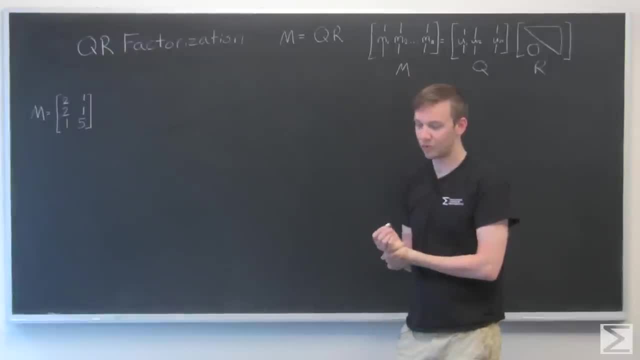 Why is this important? This has a bunch of applications with regression. When you have various points, you want to find the best fit line, But none of them really line up. This is kind of a way that you find a model that will fit to your data. So there are lots. 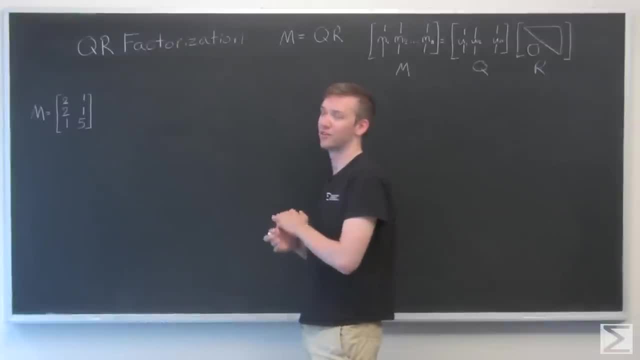 of important reasons to do this, But we're primarily concerned right now with how to do it. So we're going to use this example here, Where my M is 2, 2, 1, 1, 1, 5.. And these are going to be my M1 and M2.. So we need to 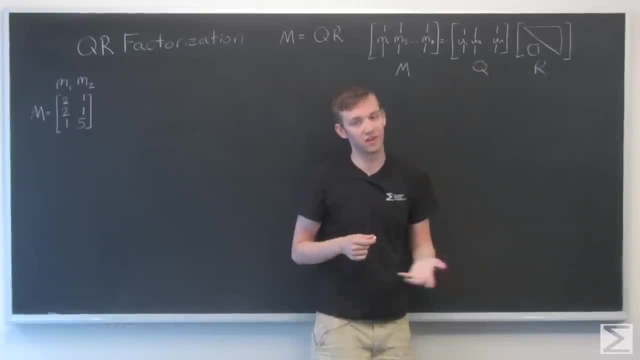 start by finding our Q, And the Q is just the Gram-Schmidt process, So we get to go through that again. Here's U1.. And that's going to equal 1 over the length of M1 times M1 itself. 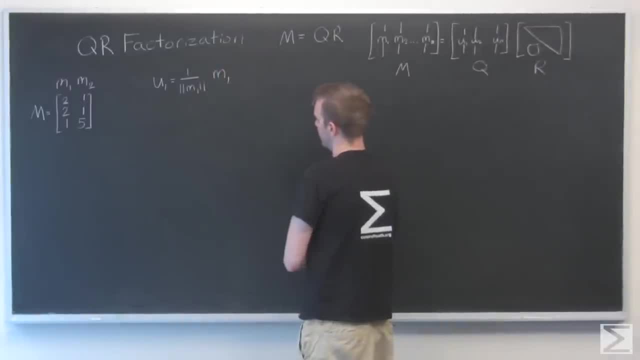 All right, And so I'll do that right now. 1 over what's the length of this? That's the square root of 2 squared plus 2, squared plus 1.. That's 4 plus 4 plus 1.. That's 9.. 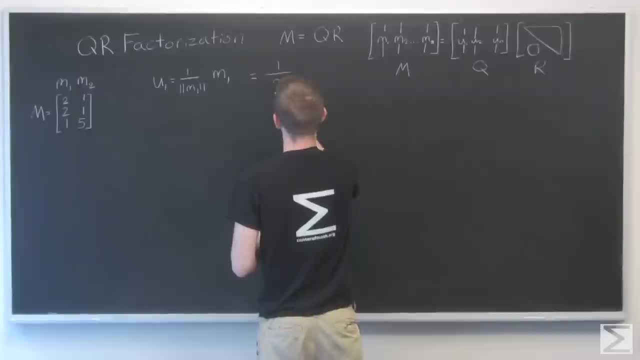 And the square root of 9 is just 3.. So 2 thirds, 2 thirds 1.. It's not unlike the example we did in our Gram-Schmidt video. All right Now U2.. Luckily, there are only two column vectors in this particular matrix. 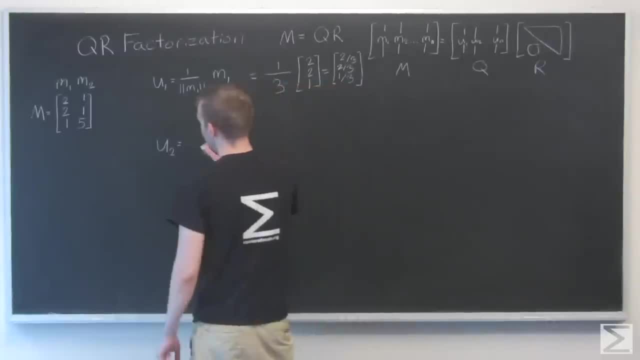 So we don't get too complicated with U3 and U4. We just have U2, which is M2 minus U2, right 1.. U1 dot M2 times U1, right OK. And then, after that's done, we're going to have to divide by its length again. 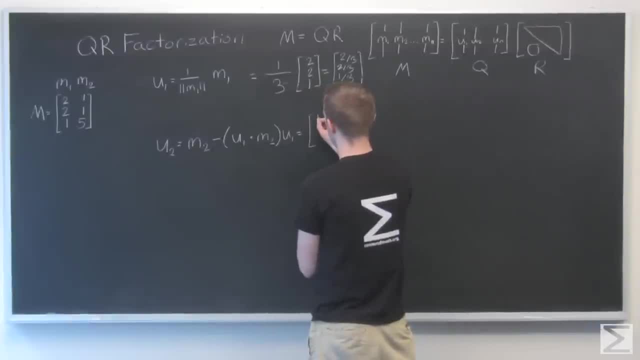 So M2 minus OK, U1, dot M2.. That's going to be OK. 1 times 2 thirds. So 2 thirds Plus 1 times 2 thirds plus 5 times 1 third, That's 5 thirds, parentheses times U2.. 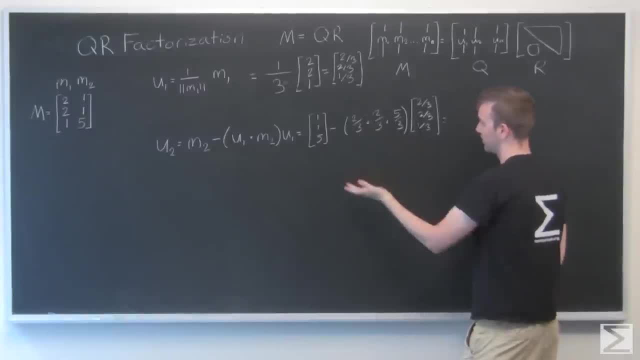 And that equals 2 plus 2 plus 5.. That's 9.. 9 thirds is 3.. So that's 1, 1, 5 minus 3 times this. OK, This is going to be 3.. 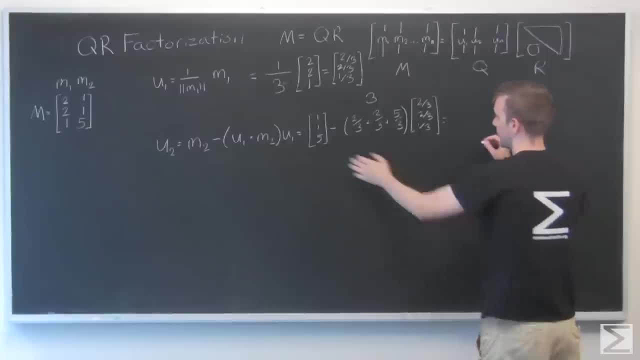 So 3 times that that'll just knock out the thirds on each one. So it's really: 1 minus 2 is minus 1.. 1 minus 2 is minus 1.. And 5 minus 1 is 4.. 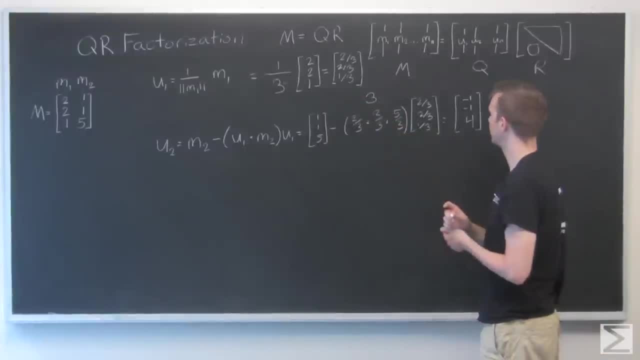 Great, That is my U2.. That is my U1.. Sorry, that is not my U2.. I forgot the last step, which is divide by its length. OK, So my real U2 is going to be: OK, 4 squared is 16 plus 1 plus 1.. 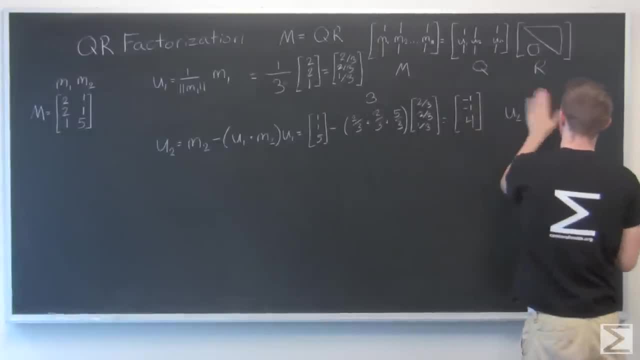 That's 18.. So not the friendliest of numbers, but the square root of 18 times minus 1, minus 1, 4.. And unfortunately, when you're doing Gram-Schmidt or QR factorization, you do get a lot of square. 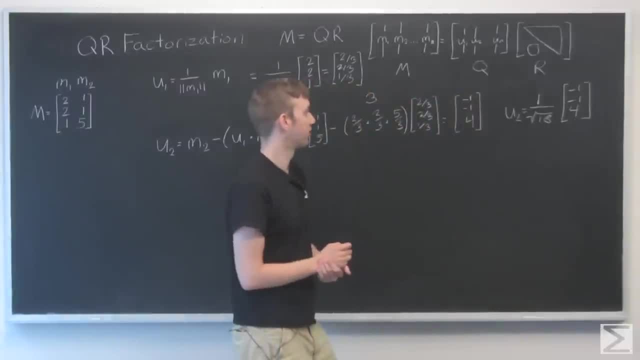 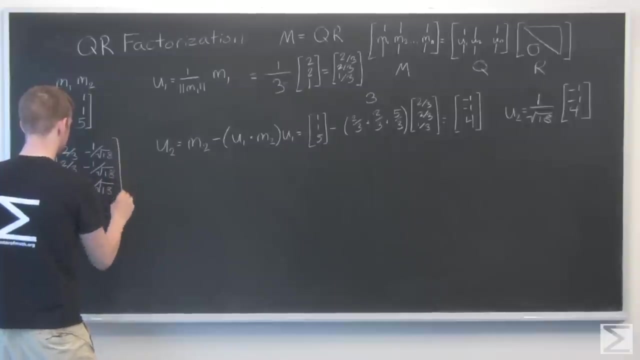 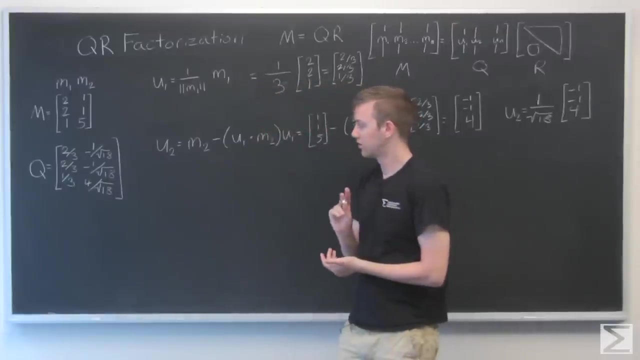 roots, because we're dealing with the hyperbolic, We're dealing with a constant, We're dealing with a penalty unit vectors. So that is my U2.. That is my U1.. I can now write my Q. OK, Right now you're probably wondering how do I get my R? And there are actually two. 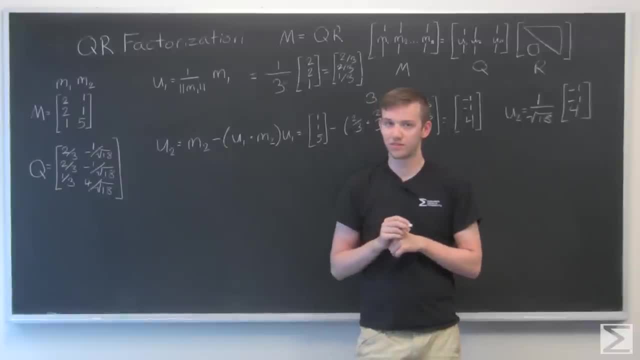 ways that you can get this. One of them is the smart way. I like to call it, But it requires you to really look into these things and think about it deeply. And if we do it the smart way, we realize that we've actually kind of already calculated R, And I'll explain what. 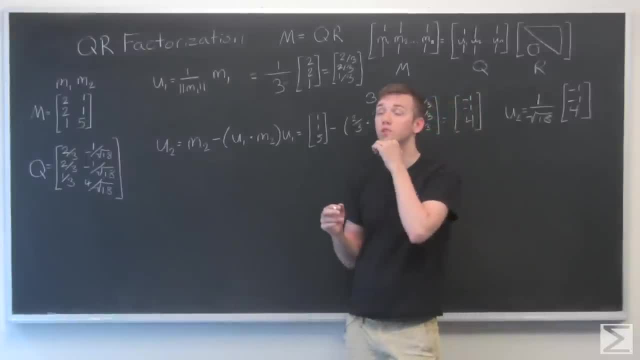 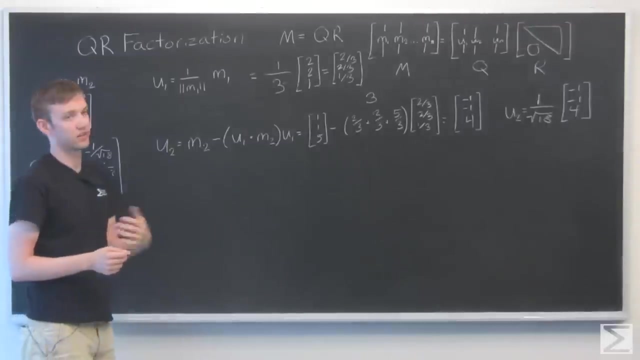 that means. And then there's more of a brute force method, which is: we've already found our Q, We've already found our M, So to find our R, that's the same as if we solve for R in that equation by multiplying both sides by Q- transpose, And our Q transpose Q, because that is an. 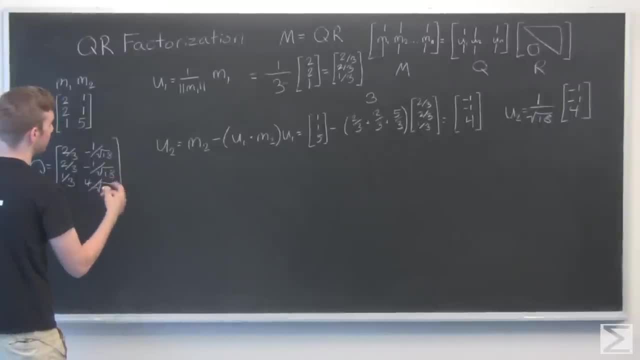 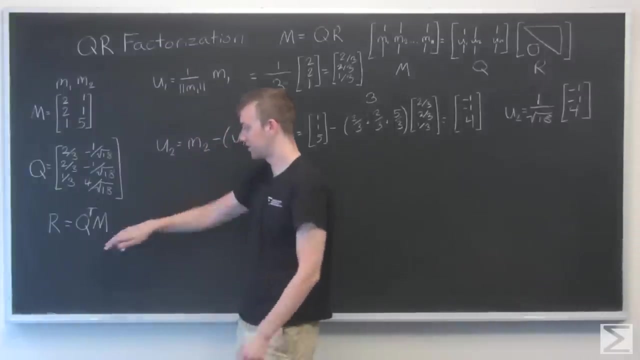 orthonormal matrix that'll give us just the identity matrix I. So R will equal R, So R is just Q transpose M. So we could multiply these matrices out, And I'll do that last to just prove that that is correct. But here's what I mean when we've kind of already calculated R. 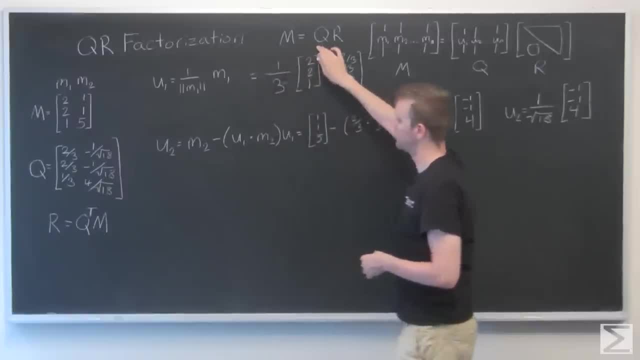 OK, First of all, M is a 3 by 2 matrix, Q is a 3 by 2 matrix, So we know that R has two to be a 2 by 2 matrix in order for us to get M. So we just had a source matrix again and we're slightly estad ceramics. So we'll see. what will happen when I get. So what I can do is I can use the Y matrix to gather all of our Y entries And we can change that matrix two by 2.. So we know that R has to be a 2 by 2 matrix in order for us to get M. 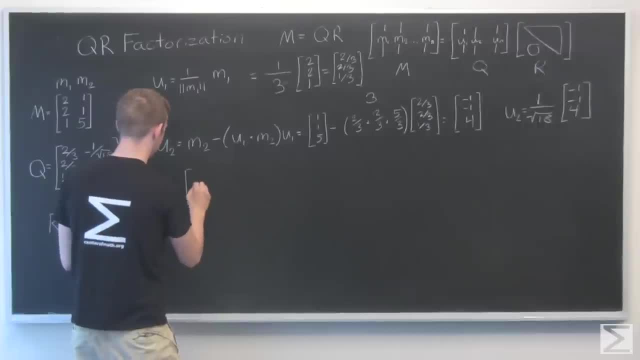 One or two by 2.. So we had Q, which was U1, U2, times some 2 by 2. matrix R, I'm going to say R1, R2, R3, and R4 equals our M1 and M2.. 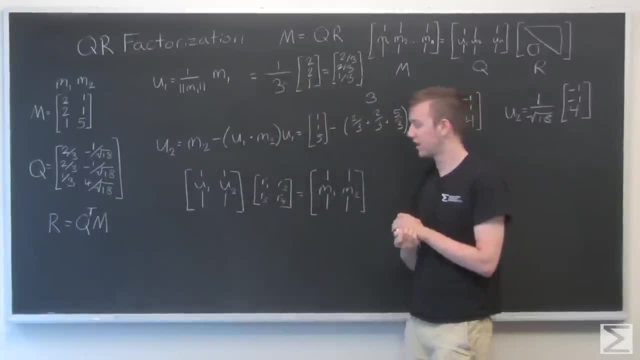 Okay, And let's think about what actually we're doing when we're doing matrix multiplication. We multiply row by column, So there are three entries here. There are actually three rows, but you don't really need to know that We multiply this first row by this first column to get this number. 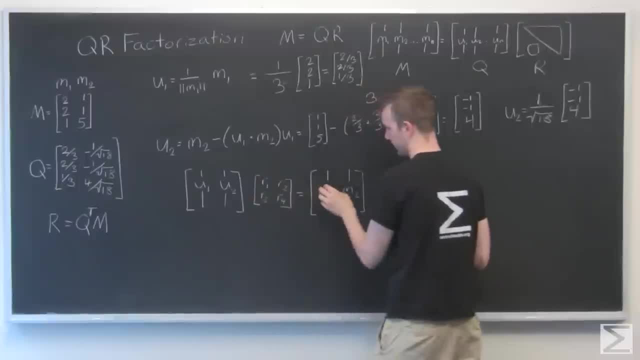 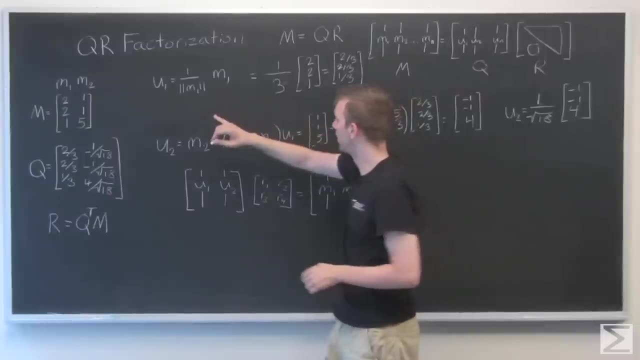 We multiply this second row by this first column to get that number. And we multiply this third row by this first column to get this number. Now, if we look up here at what we did right there, we found that U1 equals 1 over the length of M1,. 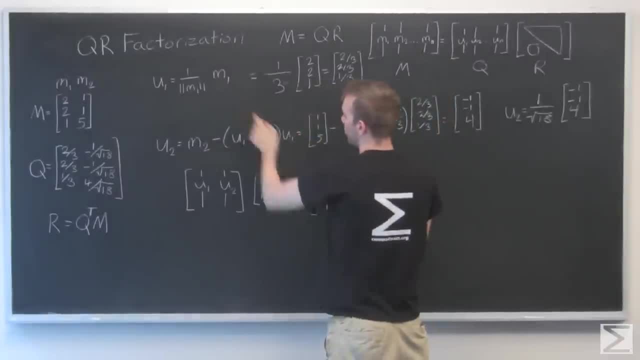 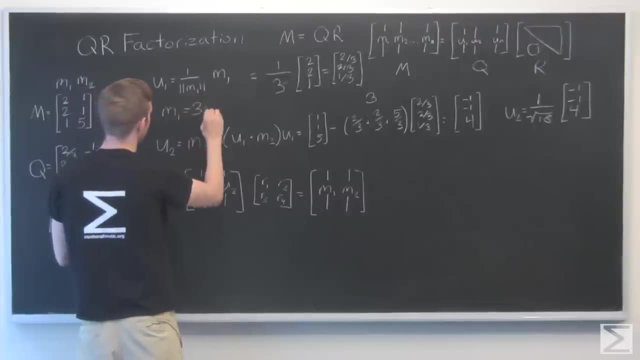 which turned out to be 3, times M1.. So from that we know that M1, this is 3.. So M1 equals 3U1.. So what does that tell us For our matrix R? that actually tells us about the first row. 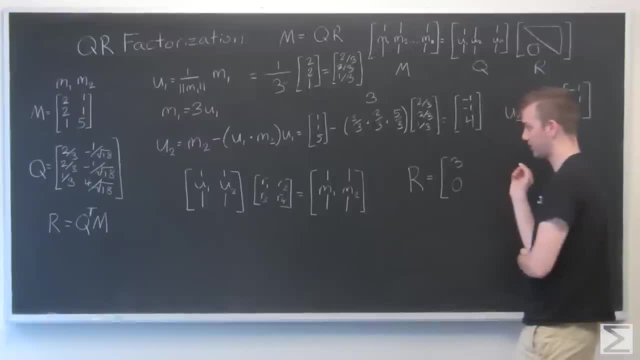 We've got a 3 here and a 0 right here. It takes a little bit of thinking and understanding to understand that. But right, this row here, which is three numbers- 1, 2, 3, results from 3 multiplied by each of the entries in this row. 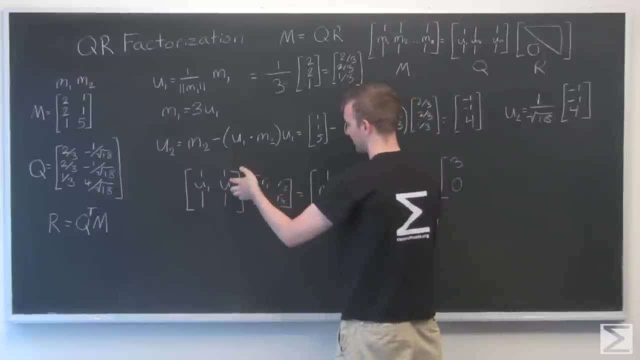 So if we multiply this by M1,, if we multiply this by M2, we're cross-multiplying each of these entries into this row. there's got to be a 3 right here in order for that to result, And there needs to be a 0 here because these numbers in the second row. 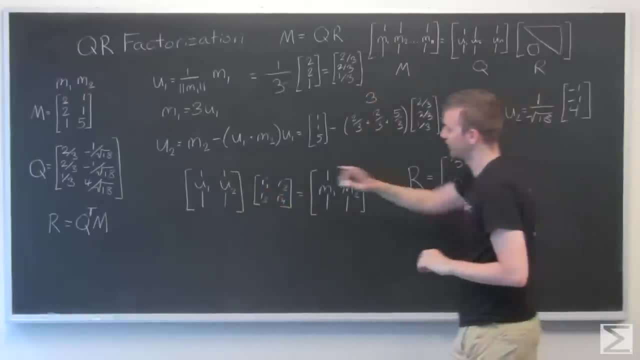 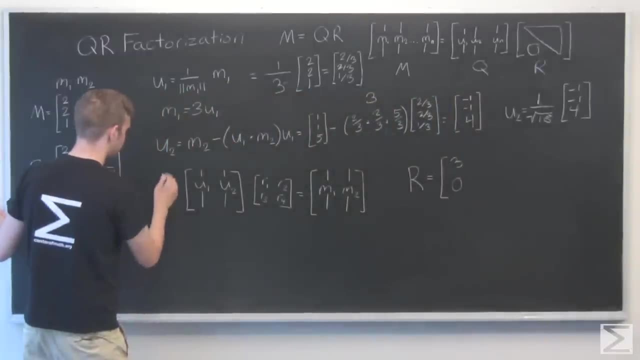 aren't being multiplied by anything. Similarly, for u2, let me just rewrite everything that we did. We found out that u2, my last step was dividing everything by the square root of 18.. And here I have m2 minus this number, which we discovered was 3.. 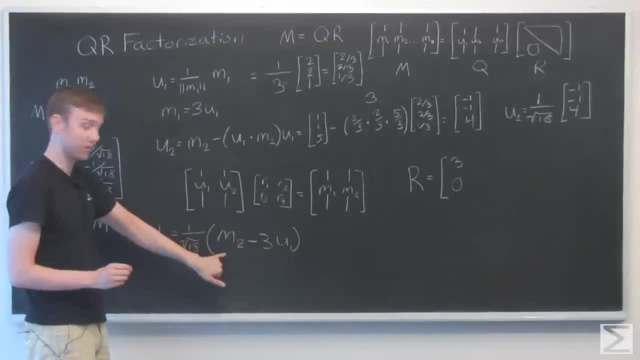 Right, OK, So let's solve for what our m2 is. If I multiply both sides by the square root of 18, I get m2 plus 3u1 plus the square root of 18u2.. So m2 is equal to 3u1 plus the square root of 18u2.. 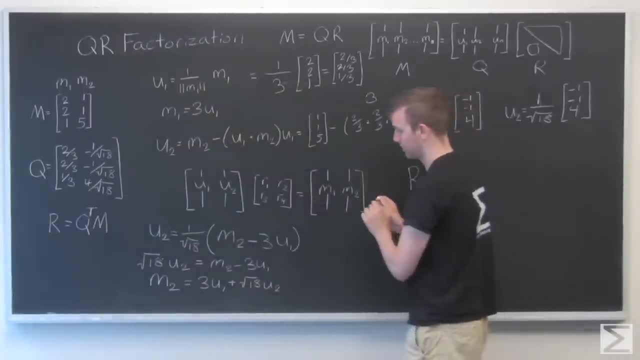 OK, So that means m2 right here is equal to when we multiply, it's all of these rows multiplied by this column right here, So all of the u1s, So all of the u1s get multiplied by 3.. 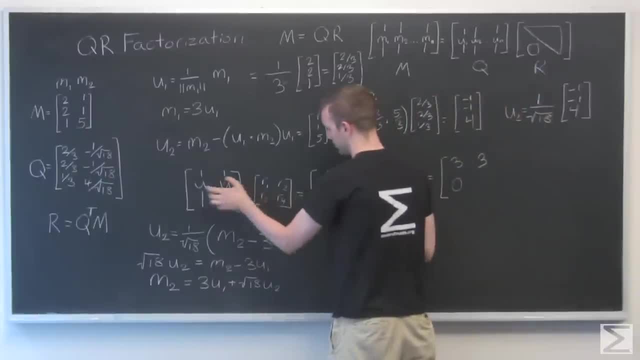 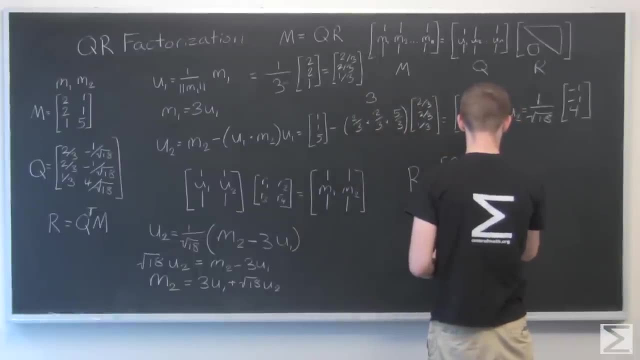 So there's got to be a 3 right there, And all of the u2s get multiplied by the square root of 18.. So there needs to be a square root of 18 right there, And that is our result r, And as you can see, we had really calculated it. 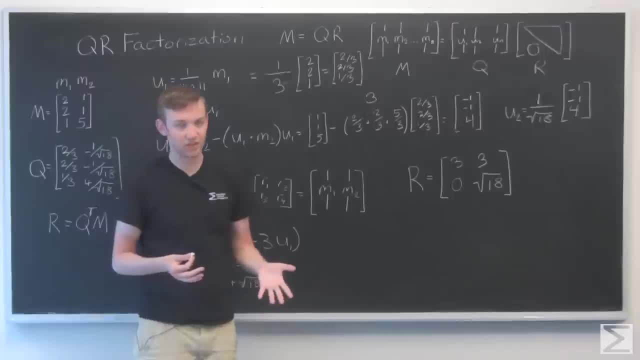 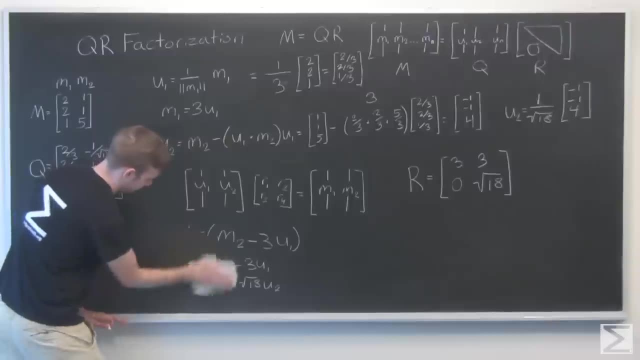 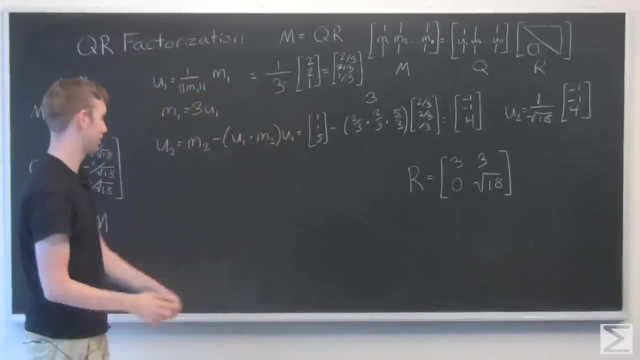 in doing this Gram-Schmidt process. That can be a little bit difficult to see, which is why I'm showing you this other method, which is easier on the brain but more work. OK, that is our answer, But we're going to just do this out. q transpose m. 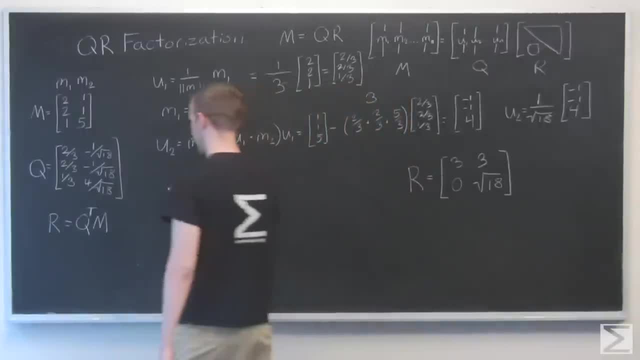 And I'll try to do this as fast as possible, because no one likes matrix multiplication. If you have q transpose, that's just shifting everything, so it's sideways. So the rows becomes the columns, the columns become the rows. So if the rows become columns, you'll 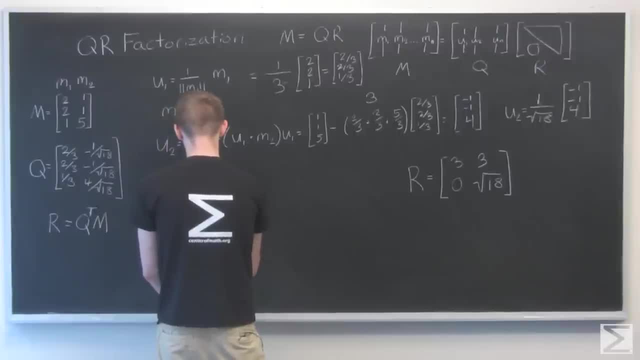 have to go from 1 to 10 to get 1.. So so I'm just going to do r transpose. sorry, everywhere the rows change. I just need to use my original energy. So 1, 2,, 3,, 4,, 5,, 6,, 7,, 8,, 9,, 10,, 11,, 12,, 13,, 13,, 14,, 15,. 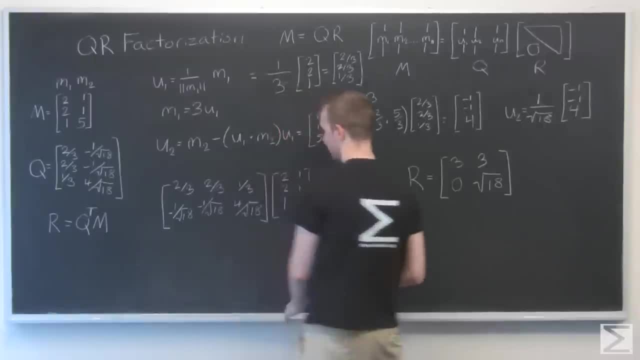 16,, 17,, 18,, 19,, 20,, 21 and 21.. Let's go to my version of the term. Let's do this, Let's do this Two-thirds times two four-thirds, Two-thirds times two, four-thirds. 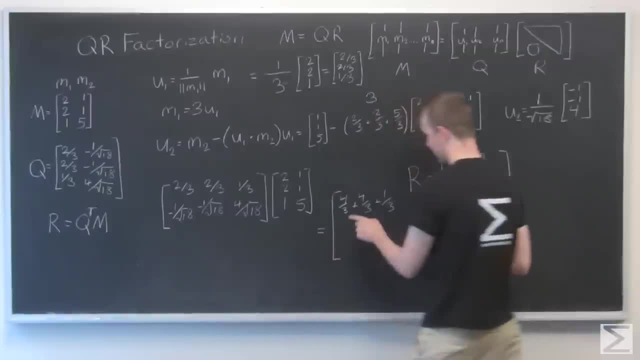 A third times one, one-third. So four-thirds plus four-thirds plus one-third. Hey, that's nine-thirds, That's three. Cool, I'm running out of room. OK, this times that We get this entry: Two-thirds times one, two-thirds. 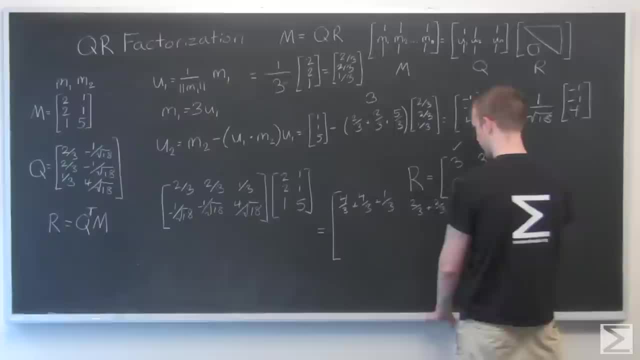 Two-thirds times one. two-thirds. Two-thirds times one-third times five, five-thirds. These are bumping into each other. I hate when I do that. But two-thirds plus two-thirds times five-thirds, That's nine-thirds. Hey, that's three. 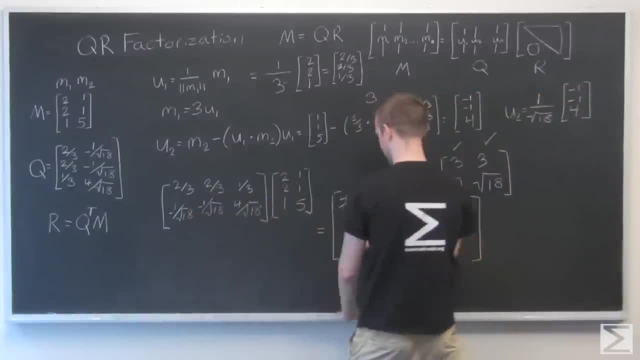 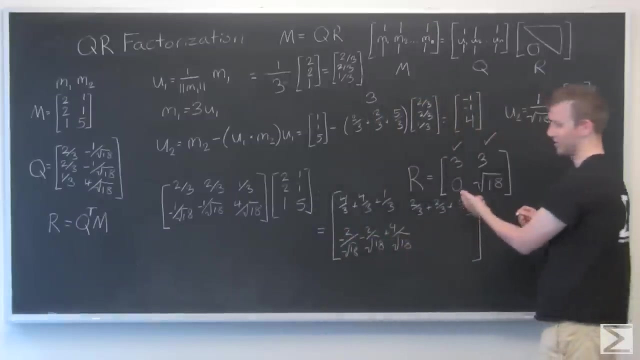 We got that right. All right. this row times that That's negative: 2, 18 over square root of 18 minus 2 over square root of 18 plus 4 over square root of 18.. Hey look, That equals to zero. 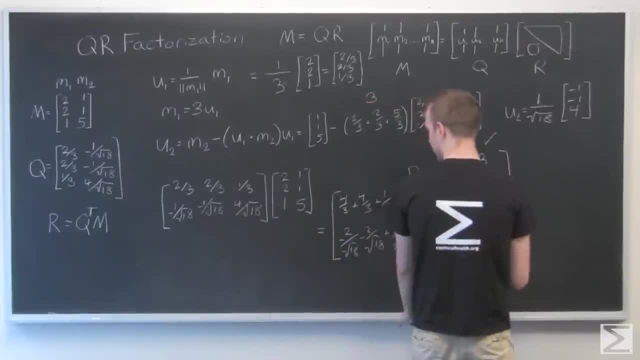 So that's right. And our last one: that's minus 1 over square root of 18, minus 1 over the square root of 18, plus 4 times 5. That's 20 over the square root of 18.. And the result of that is 18 over the square root of 18,. 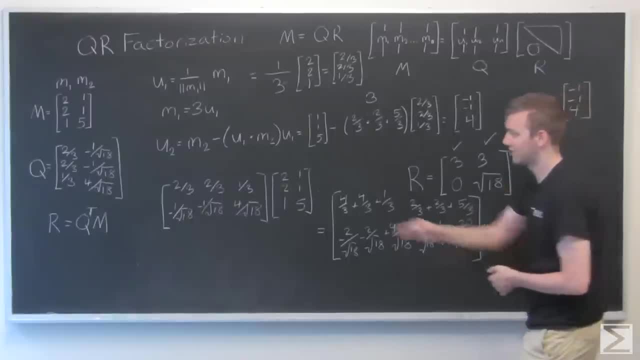 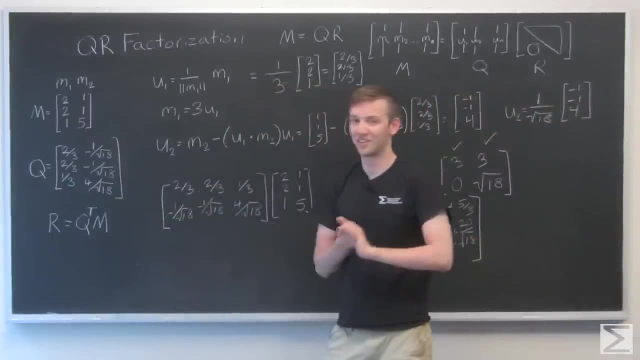 which is the same thing as the square root of 18.. So, as you can see, we got the same answer both ways. This is the method That's much easier to remember And if you aren't really in the mood to think about it. 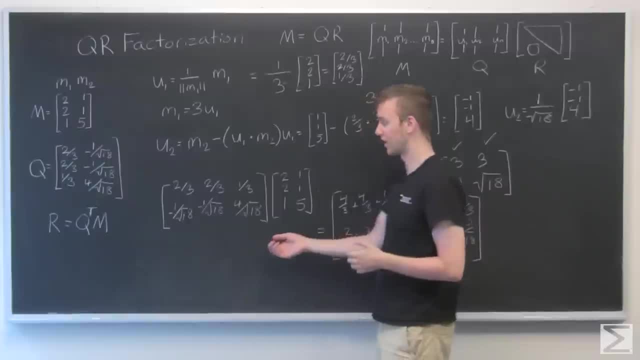 slash, less likely to make mistakes, especially if you're doing this on a calculator. I would go with that method, But it's important to understand the other one as well. So this has been QR factorization: how to divide this matrix into these two matrices. 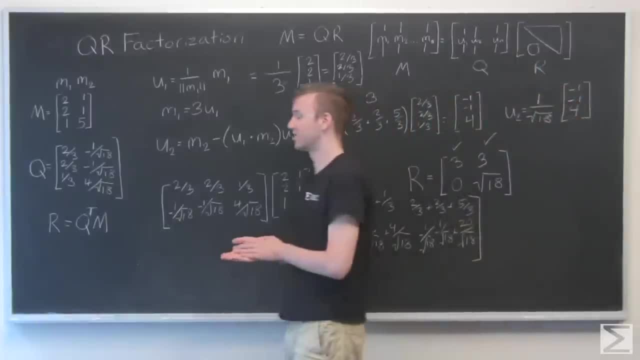 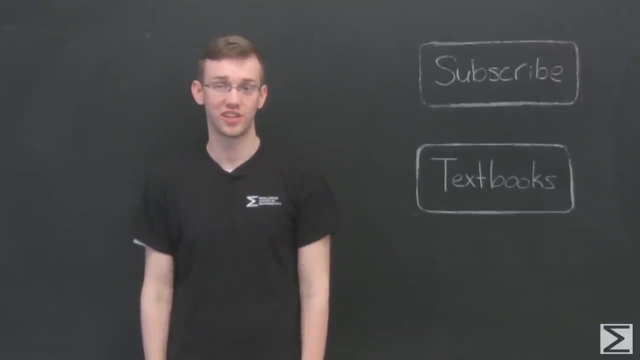 here which have various applications and things, And we just like to know how to do that. So that's all for today. Thanks for watching. Thanks for watching this video. Be sure to check out the rest of the videos in this series and any of the other math-related videos on our channel. 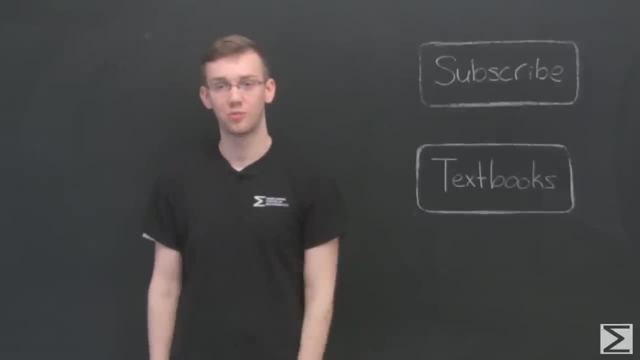 If you're not subscribed to our channel, click this link right here For more help with linear algebra. check out Worldwide Differential Equations with Linear Algebra by Robert McCohen or Elementary Linear Algebra by Bruce Kuperstein. Both are available at an affordable price.